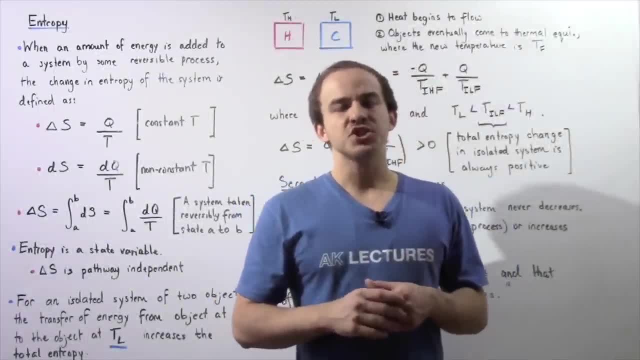 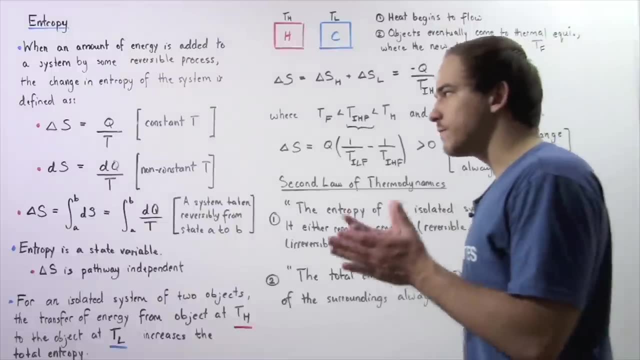 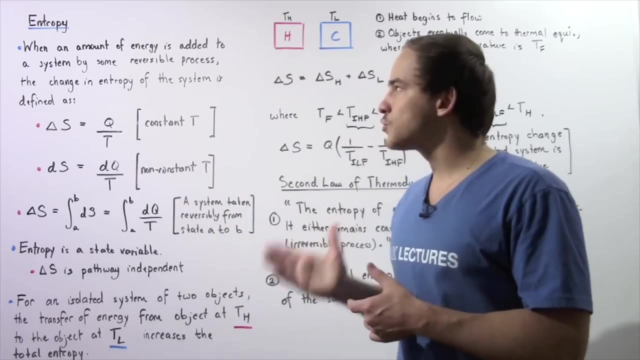 Previously, we introduced the second law of thermodynamics by stating it in a very specific way. In this lecture, we're going to discuss the general version of the second law of thermodynamics that is defined by using a concept known as entropy. Now, before we get into what the second 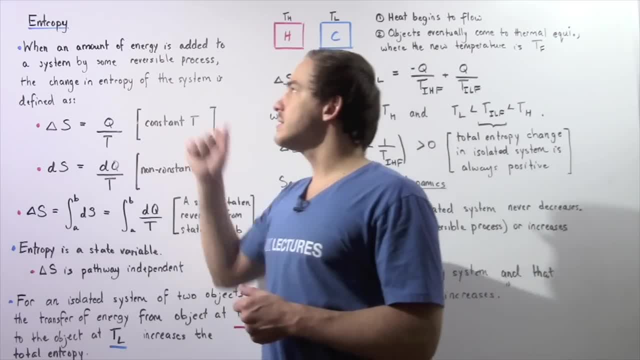 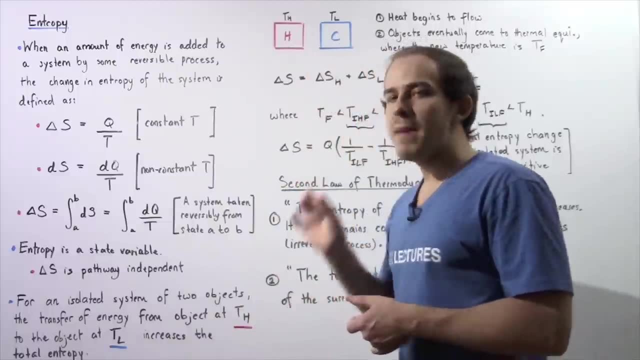 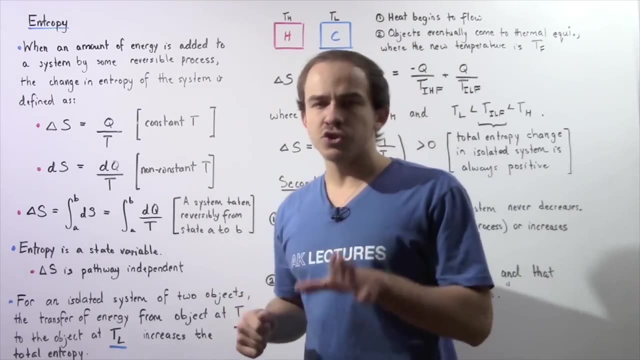 law of thermodynamics is in its general form. let's discuss this concept of entropy, what it is and how we define it. So when an amount of energy is added into a system by a reversible process, the change in entropy of that system is defined in the following way. So if our temperature is 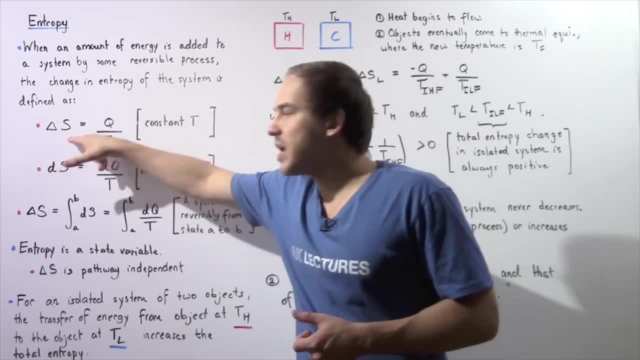 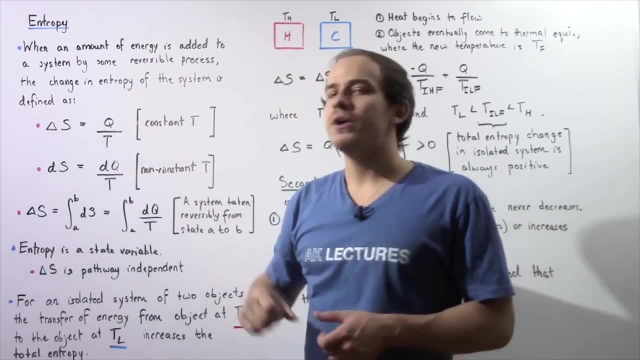 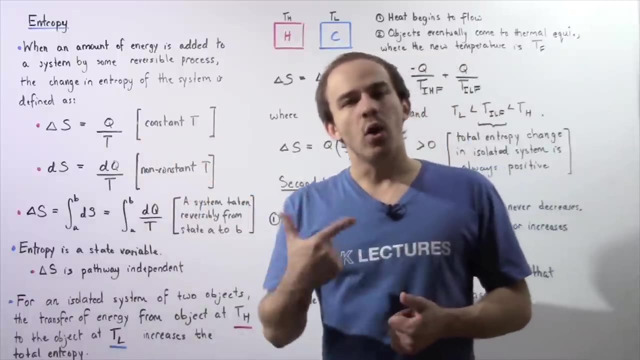 assumed to be constant during that process, then the change in entropy given by delta S is equal to Q divided by T, where Q is the energy that flows into the system And T is the temperature given in kelvins. Now what happens if the temperature during the process 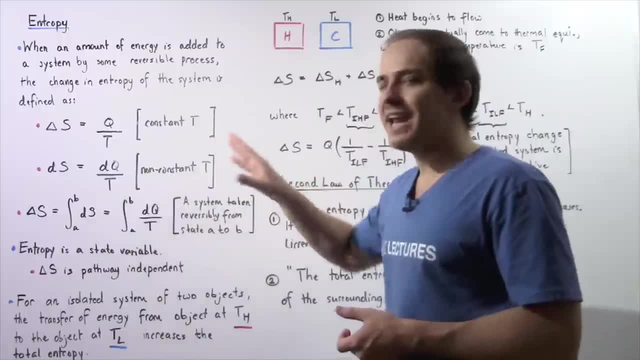 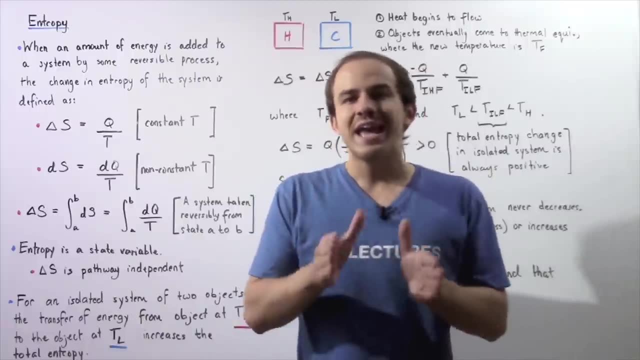 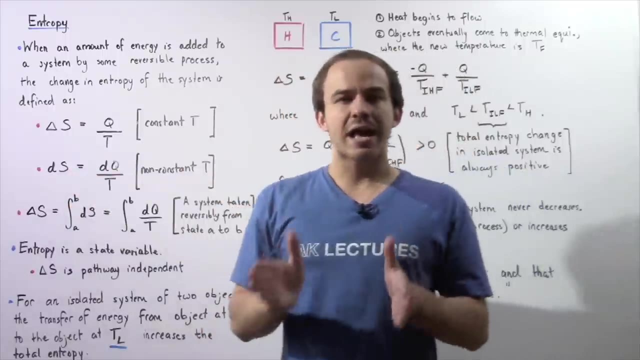 is not constant. So if we're dealing with a non-constant temperature, that means we have to talk about infinitely small changes in our entropy. So at that particular moment in time, the infinitely small change in our entropy given by dS is equal to the infinitely small. 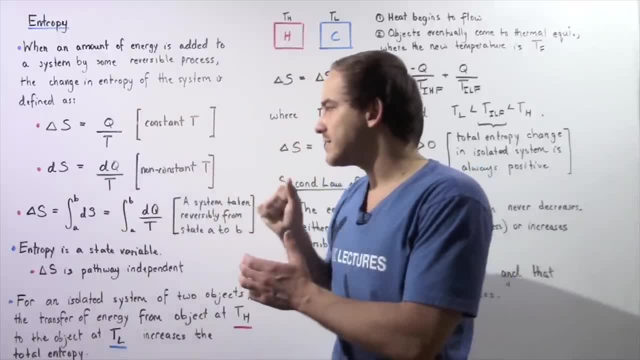 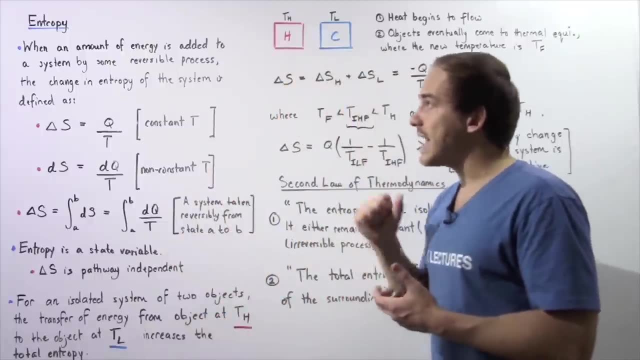 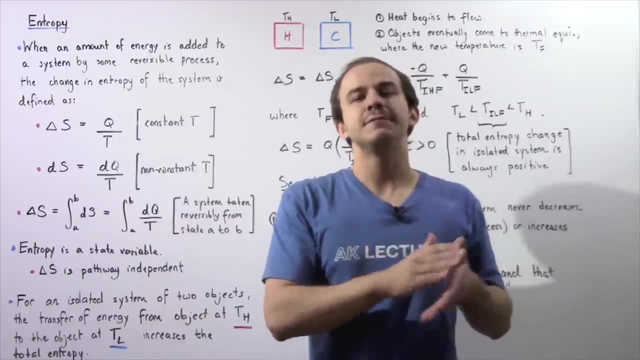 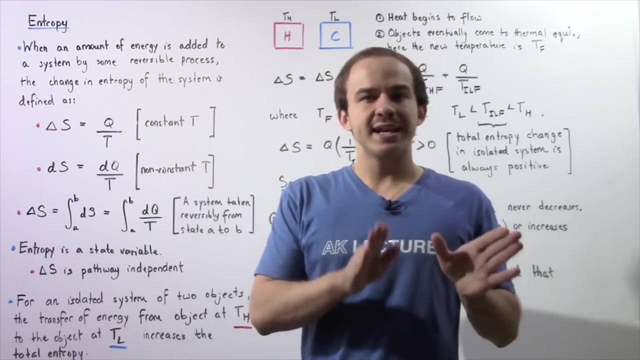 change in our energy that flows into our system, divided by the temperature at that instant in time. Now let's suppose we take our system and we take it from an initial state given at A to a final state given at B, So that means we can define the change in entropy during that process, when we take our state from A to B, in the following way: 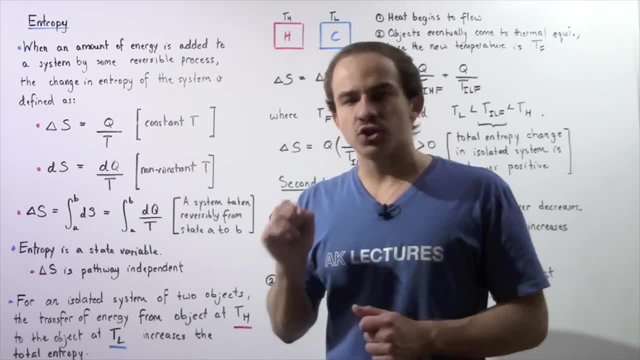 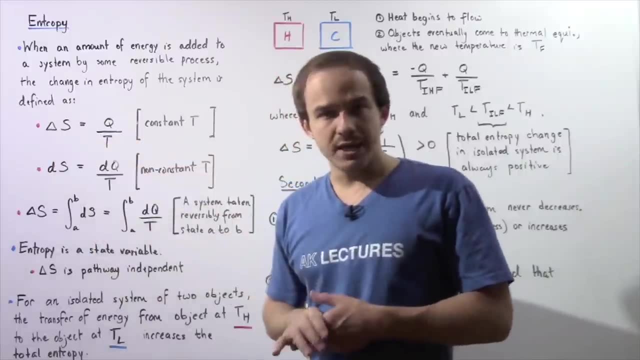 delta S is equal to Q divided by T, where Q is the energy that flows into the system. So that means we can define the change in entropy during that process, when we take our state from A to B in the following way: delta S is equal to the integral of the infinitely small change in our entropy taken from A and brought to B. 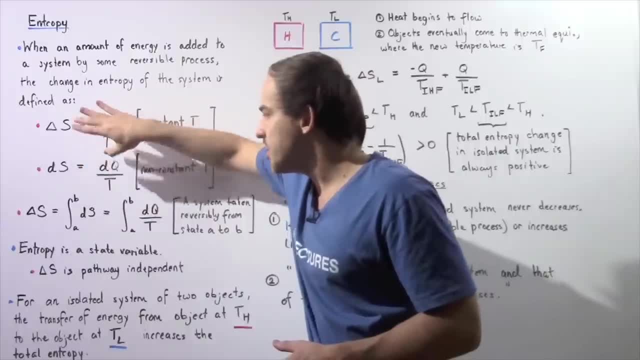 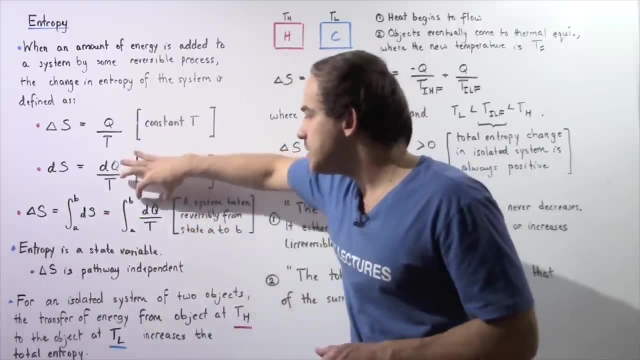 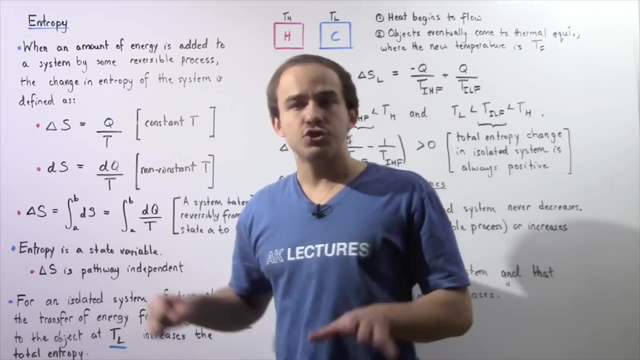 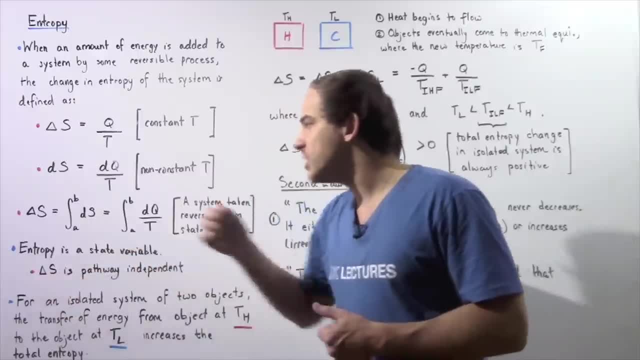 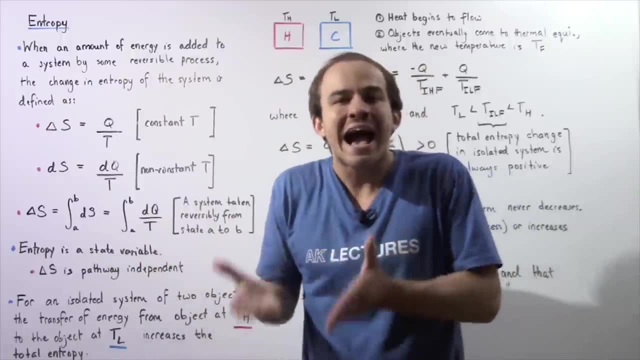 So this is our change in entropy. for a system taken by a reversal of the temperature means is the change in entropy as we go from some state A to some state B is pathway independent. It doesn't matter how we go from A to B, the change in entropy will always be the same. So 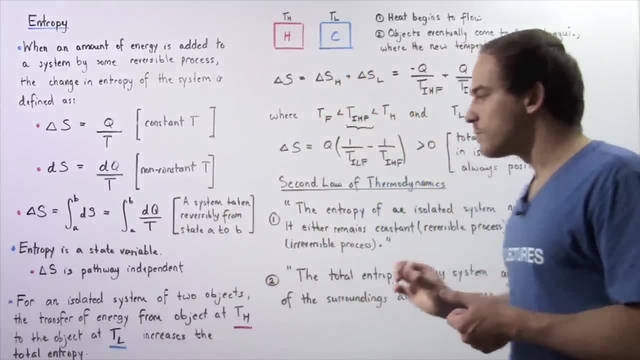 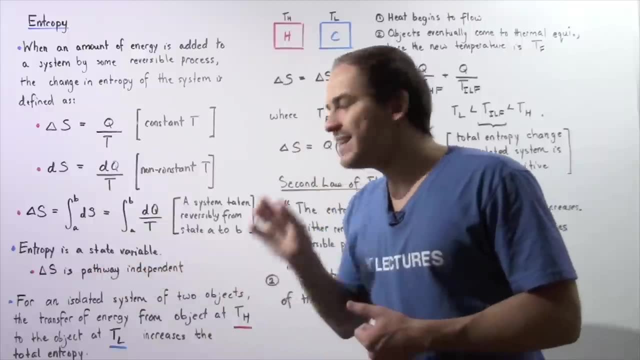 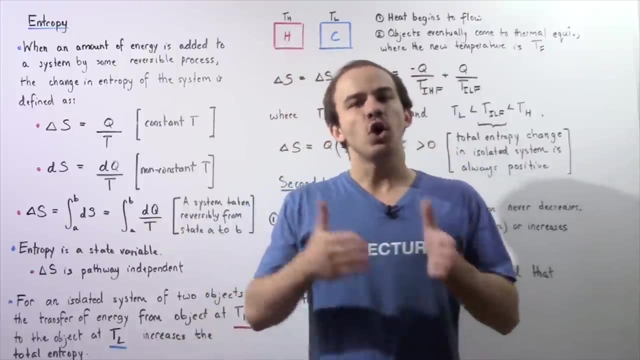 entropy is a state variable. Now let's look at the following statement and then let's see why this statement is true. So for an isolated system? an isolated system is essentially a system in which mass and energy does not flow into our system and does not leave our system. So for an 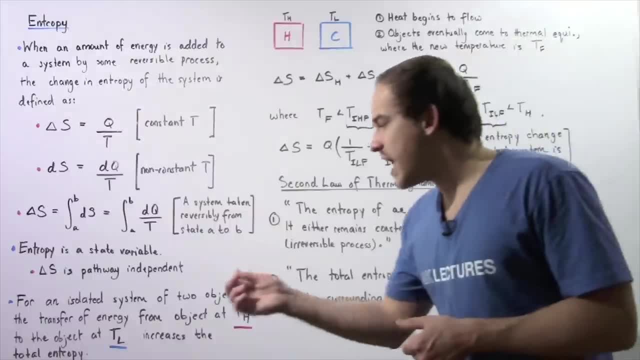 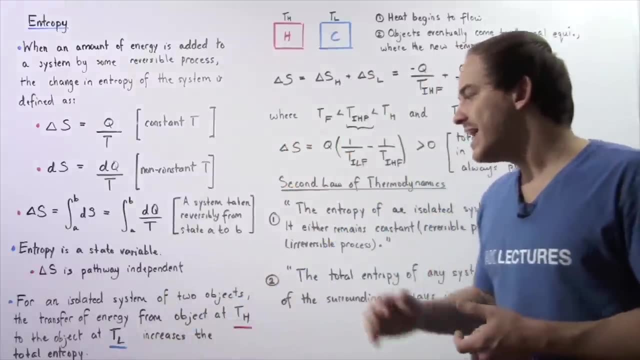 isolated system of two objects. the transfer of energy from the object at the higher temperature, TH, to the object at a lower temperature, TL, increases the total entropy of that isolated system. So for an isolated system, the transfer of energy from the object at the higher temperature, 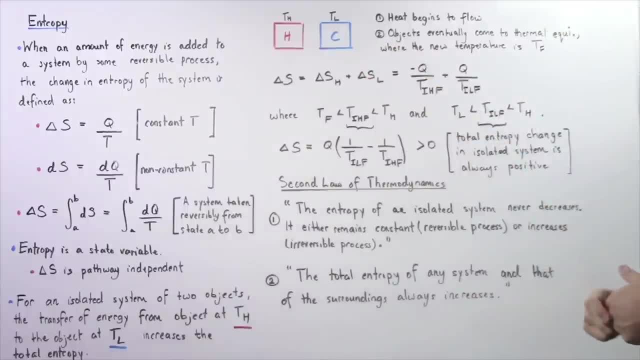 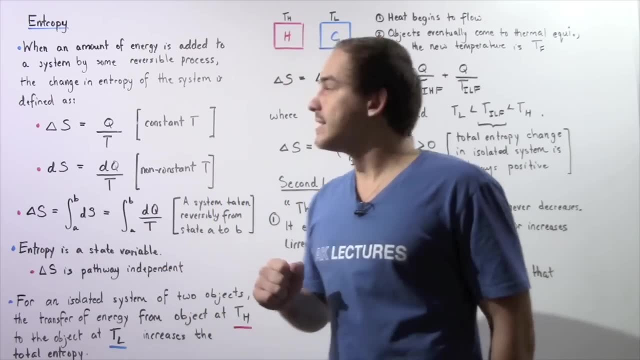 TH to the object at a lower temperature, TL increases the total entropy of that isolated system. So let's see exactly why by looking at the following scenario: Let's suppose we have two objects, and these two objects is our isolated system. So we have an object given by H at a. 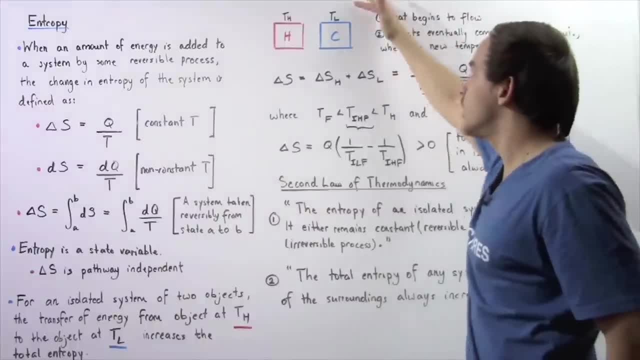 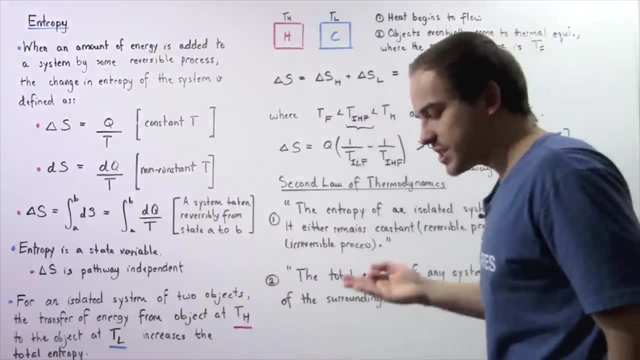 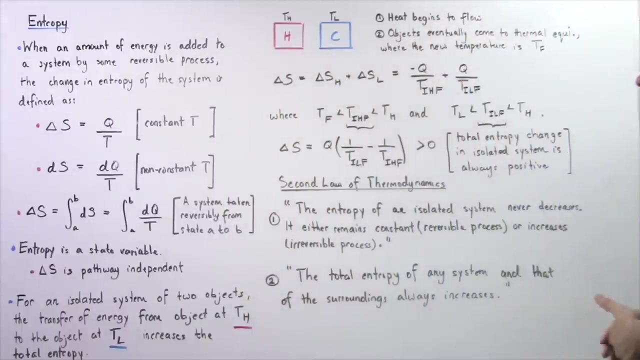 higher temperature, TH, and an object that is cooler at a lower temperature, given by TL. Now, initially, energy begins to flow as a result of heat, as a result of a difference in temperature. So we connect the two objects And heat begins to take place. Now the object eventually comes to thermal equilibrium. What that? 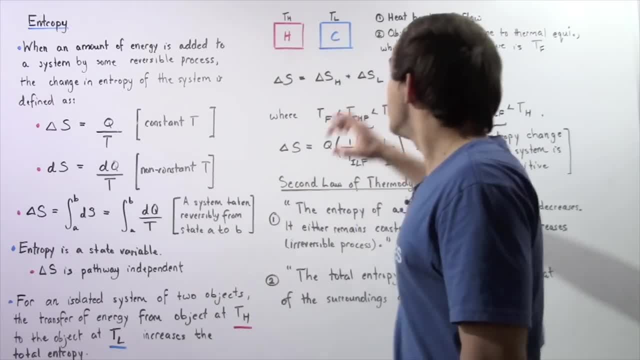 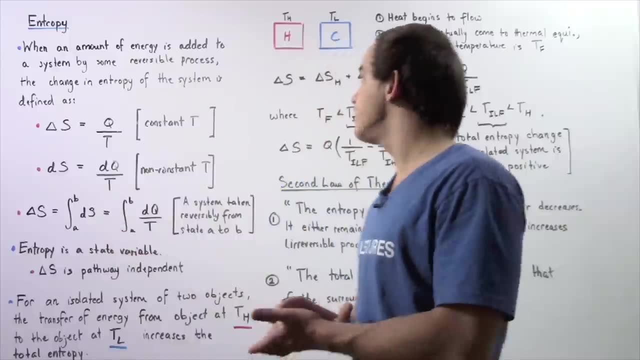 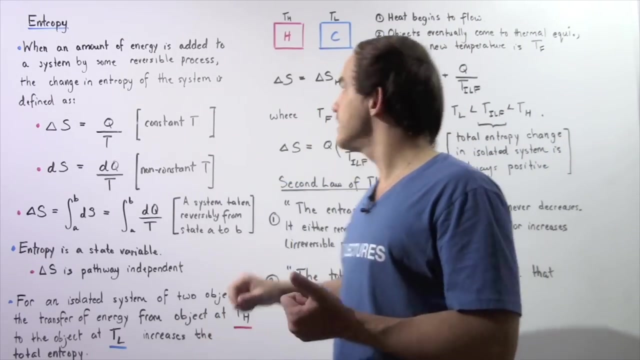 means the temperature will eventually equalize. This object will gain a certain amount of energy and this object will lose that same amount of energy. So let's represent the change in entropy of our isolated system that consists of these two objects. The change in entropy is equal to the 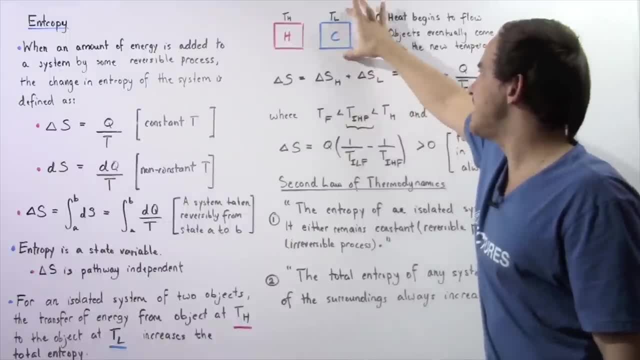 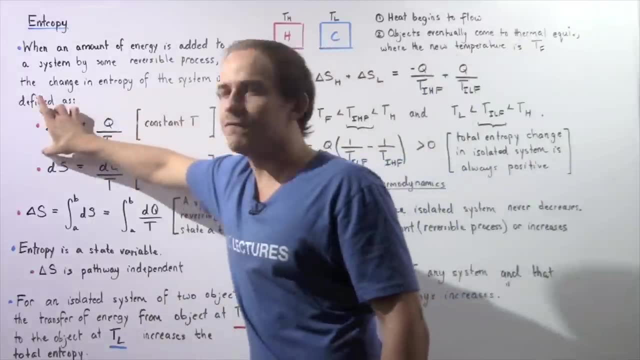 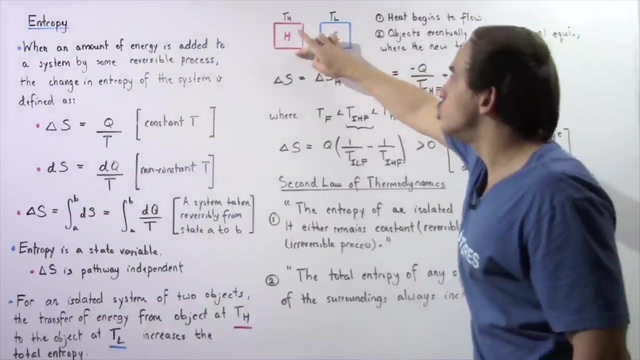 change in entropy of this object plus the change in entropy of this object, So delta SH plus delta SL. And let's go back to this formula. So the delta S is equal to Q divided by T. Now this object loses energy, and let's say it loses negative Q energy. 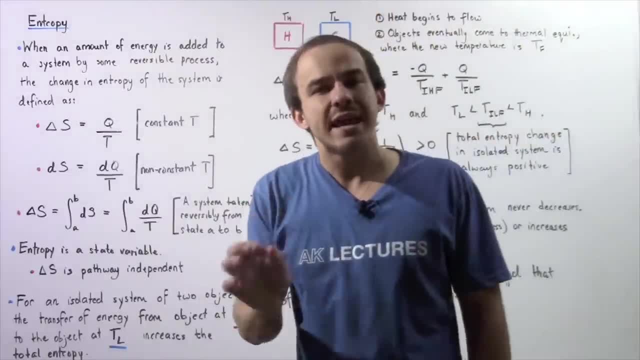 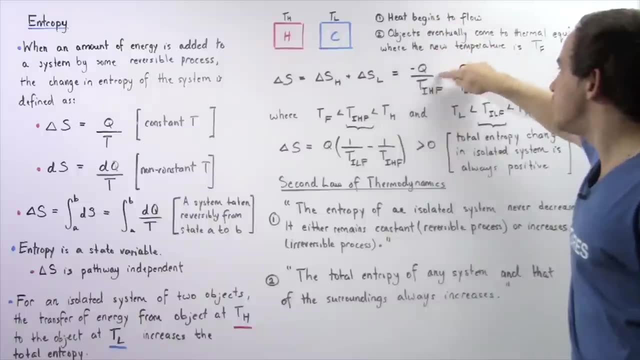 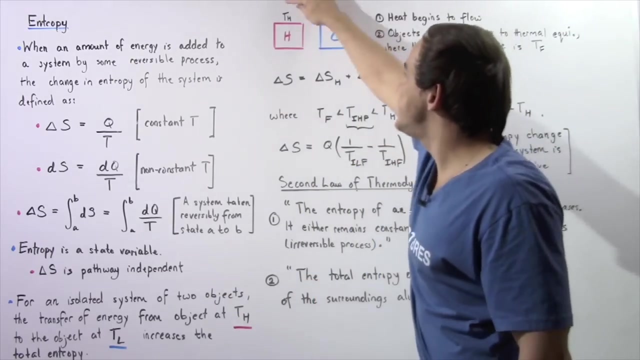 That means this object must gain that same quantity of energy, because we're dealing with an isolated system. So we have negative Q divided by this temperature, plus positive Q divided by this temperature. Now, what exactly is this temperature? Well, this temperature is simply the temperature, the intermediate temperature between TH and the final temperature. 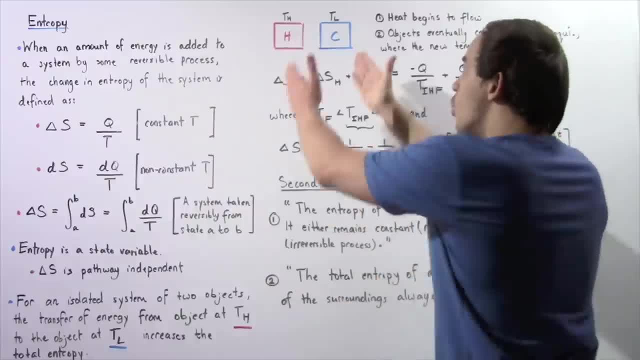 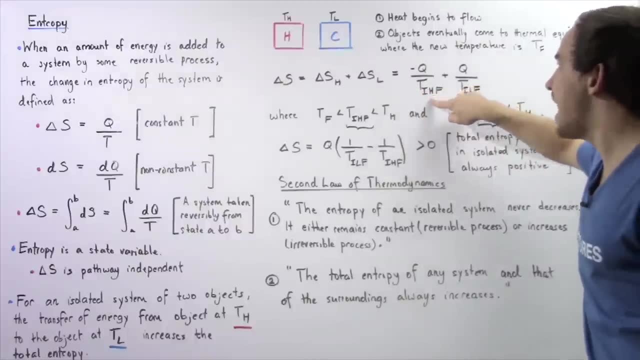 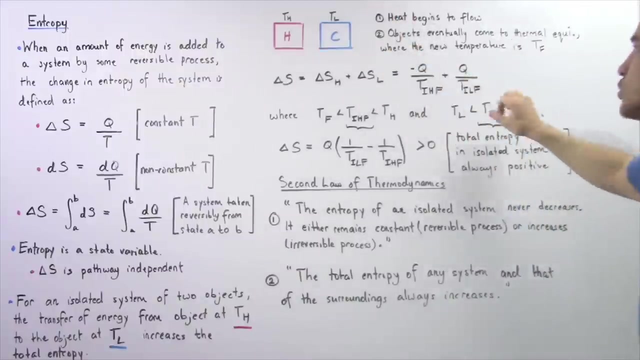 So TF is the final temperature that is reached when the object are brought into thermal equilibrium. So T, intermediate temperature between TH and TH, the H, the high temperature and the final temperature. And this is the intermediate temperature of this object between TL and the final temperature. So our range is given by the. 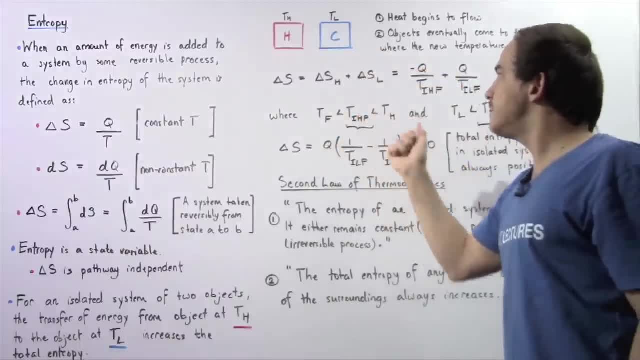 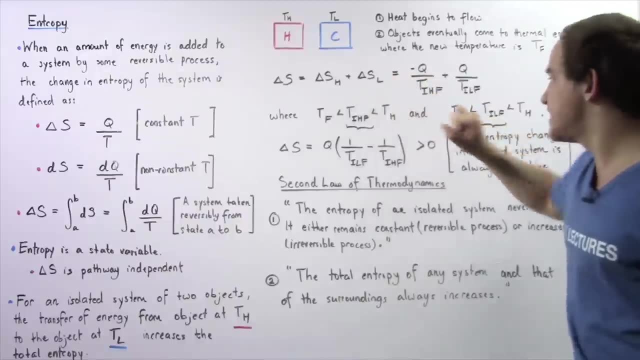 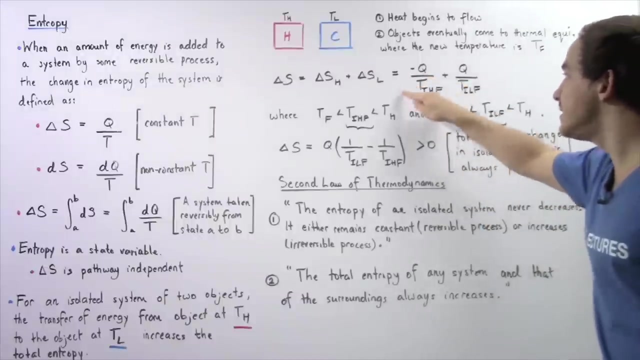 following: We have our temperature intermediate between the H and the F, for this object is between the final temperature and the high temperature, while this temperature is between the high and our low. Now notice: this quantity is greater than this quantity and this will become important. 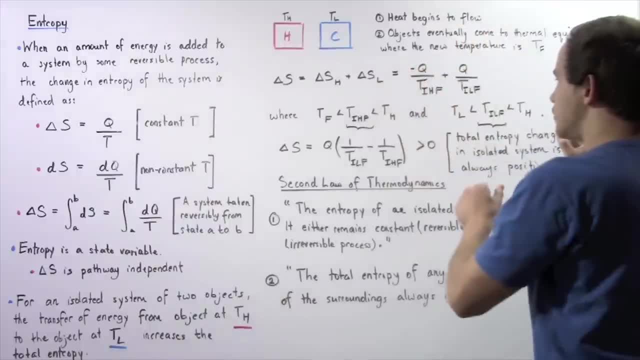 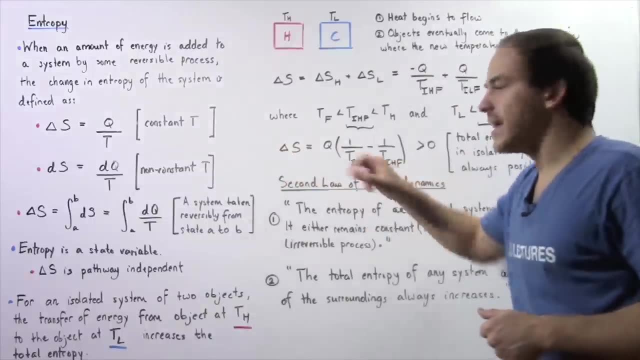 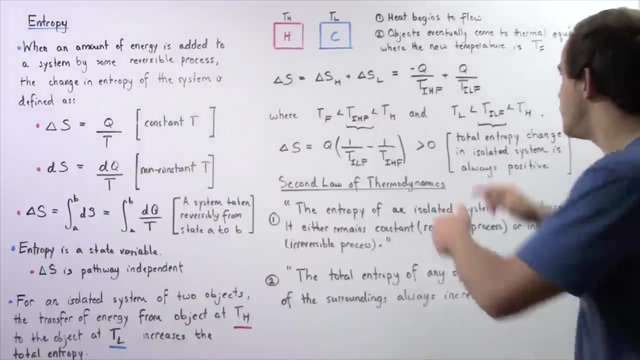 in just a moment. So let's rearrange this equation and let's take out the common term, Let's take out the Q and we get the following result: The delta S, our change in entropy, is equal to Q multiplied by the difference in the two fractions. So we simply rearranged these two fractions. So 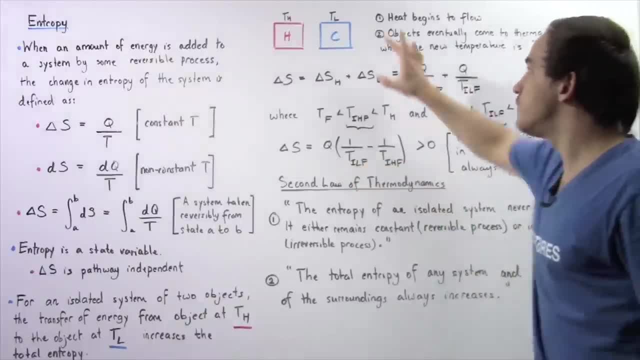 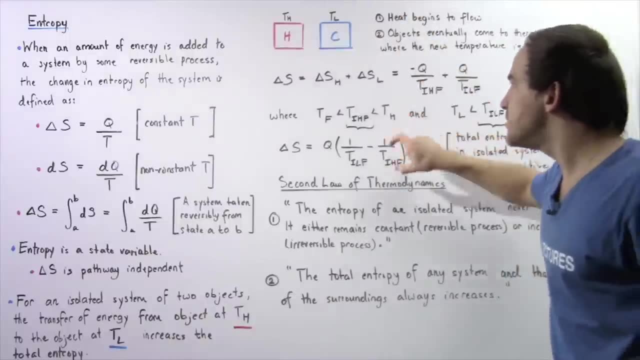 we're going to take out the common term and we get the following result: The delta S- our change in entropy- is equal to 1 divided by the intermediate temperature of this object between the final temperature and the low temperature, And this temperature is the intermediate temperature of. 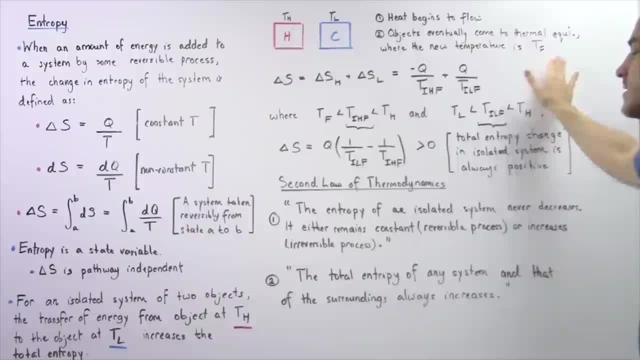 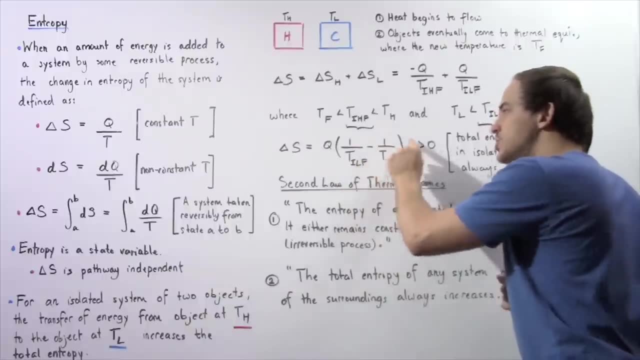 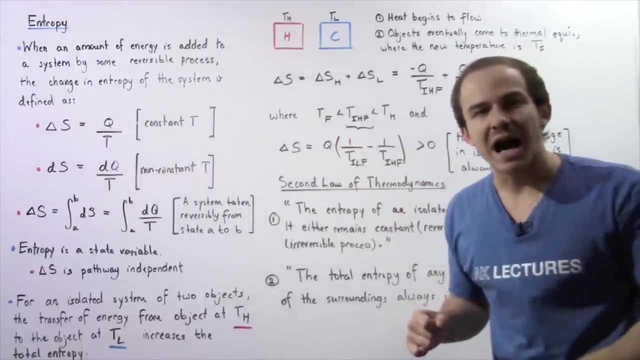 this object between the high temperature and the final temperature. Now notice: this lower denominator is greater than this. That means this fraction will be less than this fraction, So the difference of these two fractions will always be positive. So we're going to take out the common.